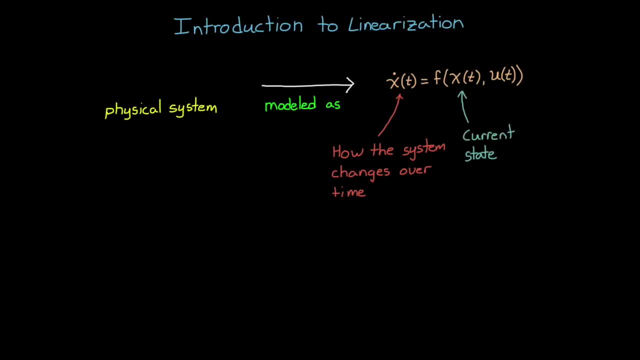 the system changes over time, depends on the current state of the system and the external inputs into the system, And this could be things like external forces and torques and energy and so on. Now, often this representation is nonlinear, since all real systems are nonlinear in nature, And the question is: can we find a? 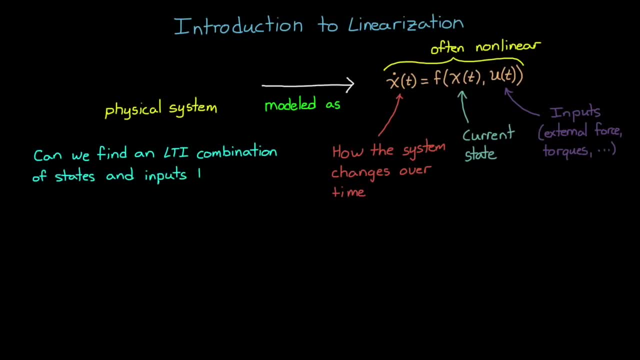 suitable linear, time-invariant combination of system states and external inputs that produce similar results as the nonlinear dynamics in some limited sense, That is, can we fit the model that is a nonlinear function of x and u to the linear form? x dot equals ax plus bu. And what are the? 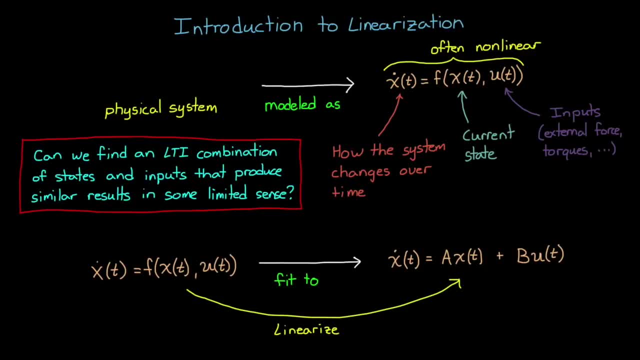 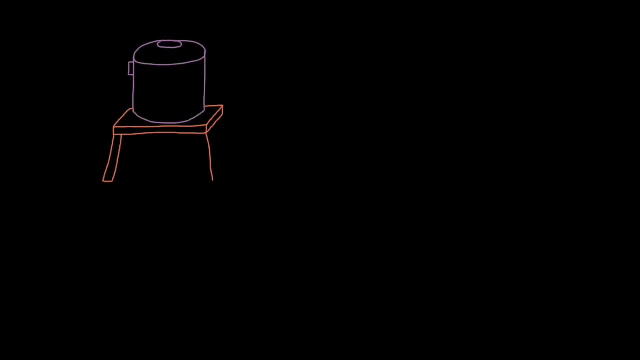 implications of doing so. Well, let's talk about that. I'm Brian, and welcome to a MATLAB Tech Talk. To begin, let's look at a MATLAB example of a water tank system. Water is pumped into the tank through an opening at the top at a rate proportional to the 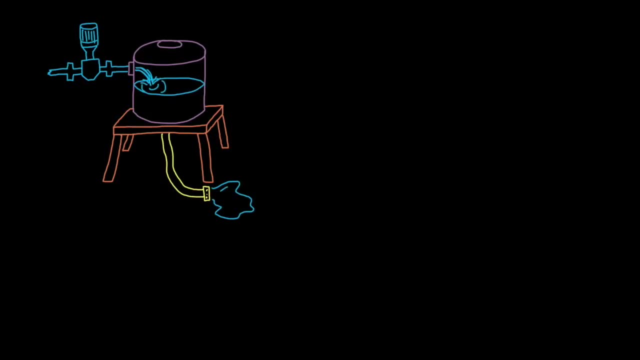 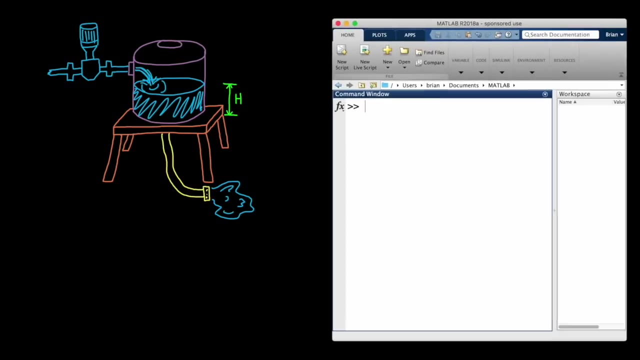 voltage that drives the pump And there's a drain at the bottom where water can leave the tank. Now the height of the water in the tank changes and can be affected by controlling the voltage to the pump. If you open up a MATLAB command window and type water tank. 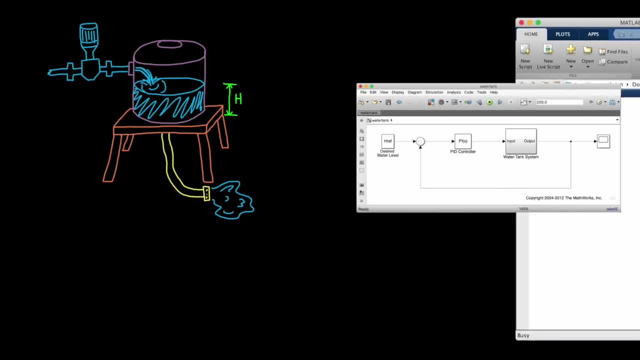 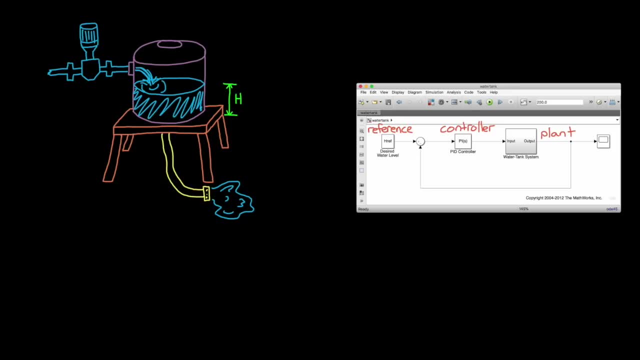 the following simulation will appear. The tank model will pop up, And this is a classic feedback system. There's a reference water height, a controller and a plant that represents the dynamics of the water tank system. The input is voltage and the output is water height. 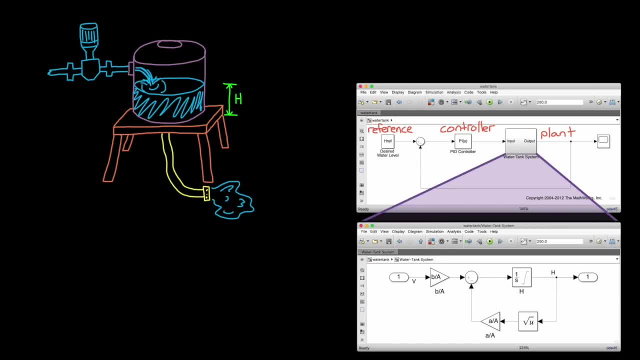 Within the plant subsystem. we have the details on how it's modeled And from this we can write out a differential equation for the system. The parameters A, B and capital A are specific parameters of the tank and they represent constants related to the flow rate. 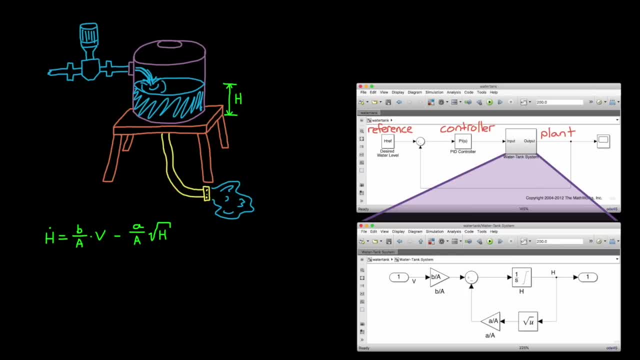 into and out of the tank and the cross-sectional area. So what we have is that the change in height of the water equals the amount of height gained by the water entering the tank minus the height lost by water leaving, And the amount lost is proportional to the square root of the water height. And this square root 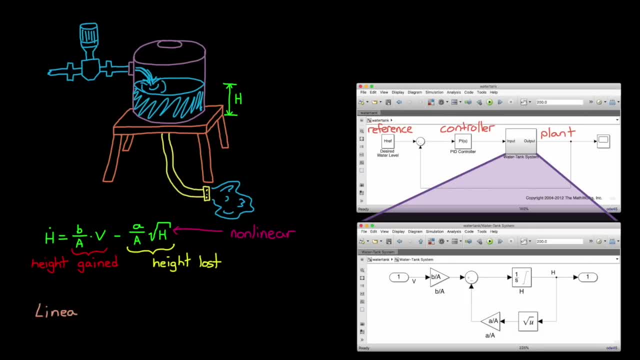 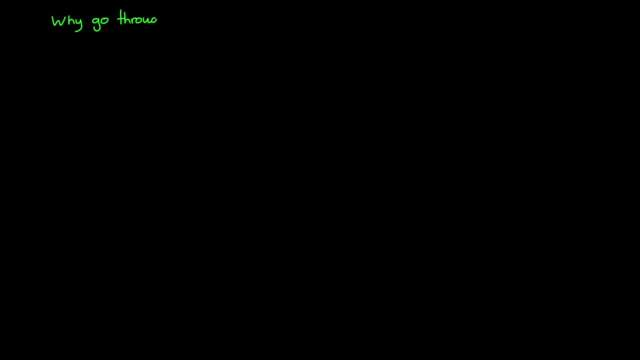 makes it a nonlinear system. So at this point we could linearize this model and fit it to the form x dot equals AX plus BU. So the question might be: why go through this process? Why go through this process? Why go through the trouble to get a linear model? Why not just stay with the more accurate? 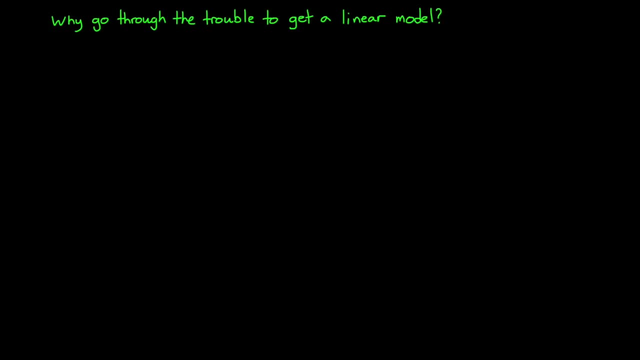 nonlinear model. Well, there's at least three good reasons. One, we can more easily check local stability and understand the dynamics of a linear system than we can a nonlinear system. Two, we have a bunch of tools that we can use to design a controller for linear. 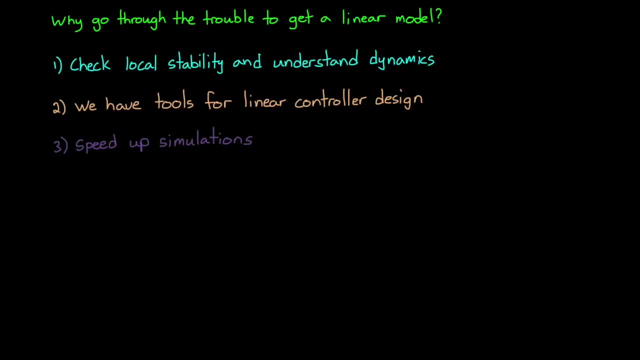 models And three. you can speed up your simulation by replacing the nonlinear model with a linear one, And this might be important if you're running a hardware-in-the-loop test, where your controller is running on the target hardware but it's interacting with a simulation. 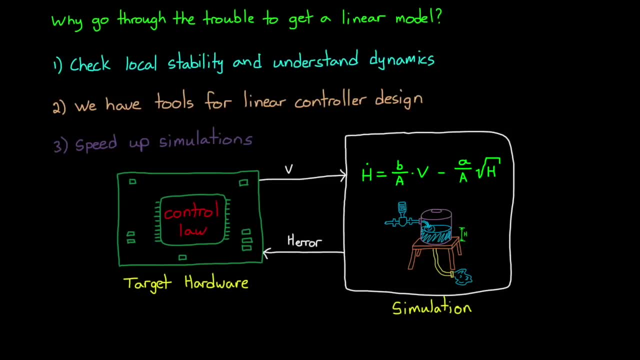 of the rest of the system dynamics. In some cases the nonlinear math involved in running that simulation can't be solved fast enough to keep up with the real-time hardware, So replacing it with a faster linear equivalent is a good option. So with that in mind, let's 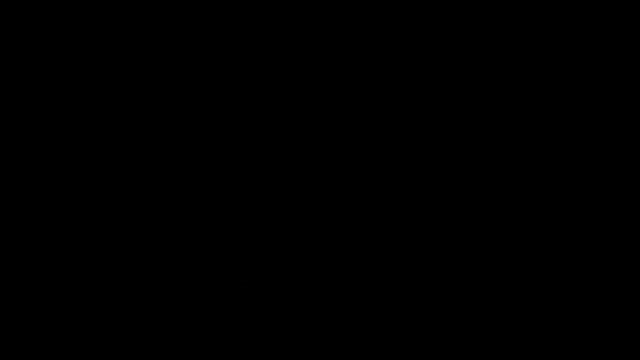 get into the process of linearization. At any moment in time a dynamical system has a state, That is, a particular configuration of system variables that define the condition of the system- Position, velocity, voltage and so on- And this set of all possible configurations that a system can be in is called the state. 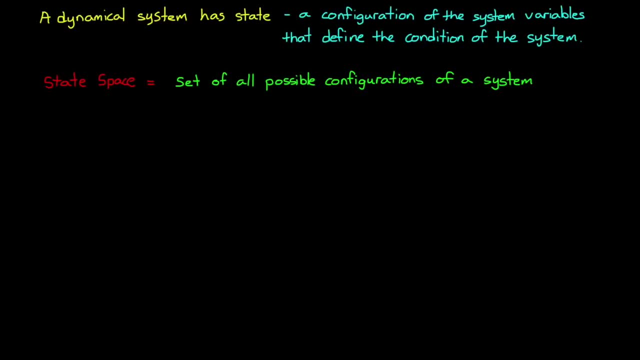 space. This is every single orientation, motion and condition that a system can experience. For example, take a pendulum that has two states- angle- theta- and angular rate- theta dot. The state's space would stretch from zero to two pi for theta to cover the entire. 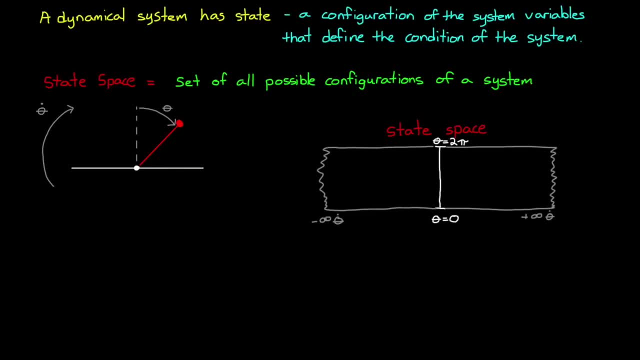 circle, negative to positive, infinity for theta dot to cover all possible rates at which it could spin. Now, of course, realistically your pendulum might never exceed something like 10 radians per second, so we can chop it down to this much smaller operating state space or the operating envelope. 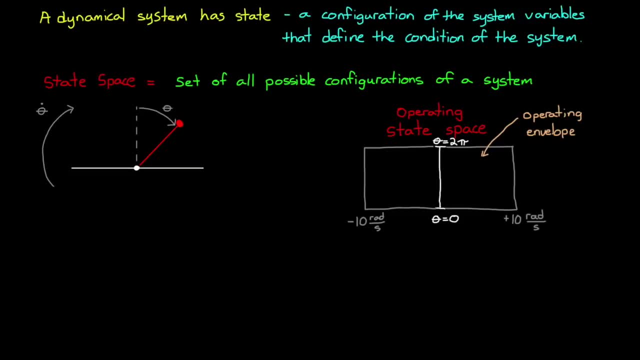 It would be ideal if we could just get a linear model that worked well over the entire state space, but that usually isn't the case, because a single linear model might represent the dynamics well at some states but due to the non-linearity of the system, it would be a poor representation at others. 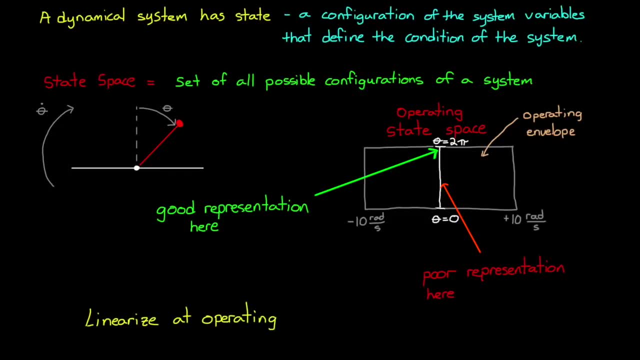 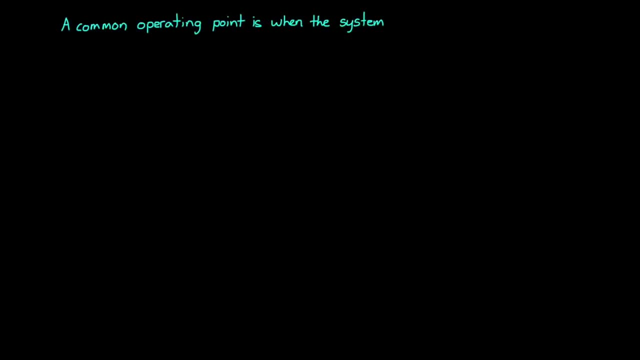 so, to work around this, we linearize at specific locations, called operating points, where we want the lowest error. Now, an important and very common type of operating point is when the system is at steady state or equilibrium. This means that if you initialize the system at this state, 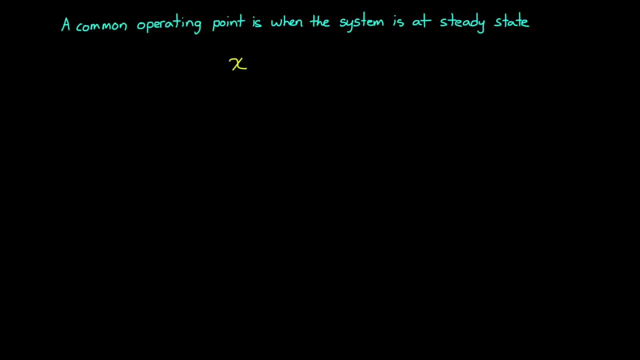 then the states would not change over time. or another way of putting it: x dot for all time equals zero. That might mean that the system states are at an equilibrium on their own with no external inputs, like a pendulum that has two equilibrium points, one hanging straight down and one perfectly. 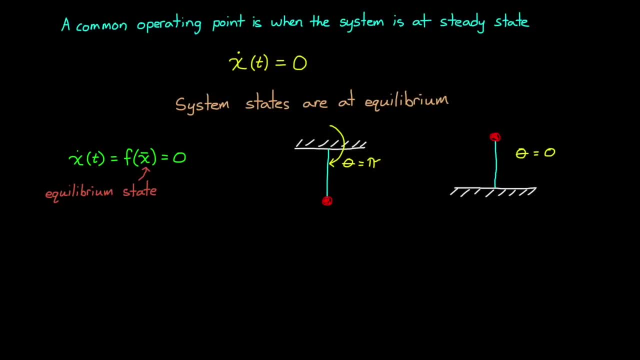 balanced, pointing straight up. but we also have inputs into the system and the combination of inputs and the system states can also be at an equilibrium. For example, if the input into the pendulum is a torque, then we can find a constant torque that moves the equilibrium point to pi over. 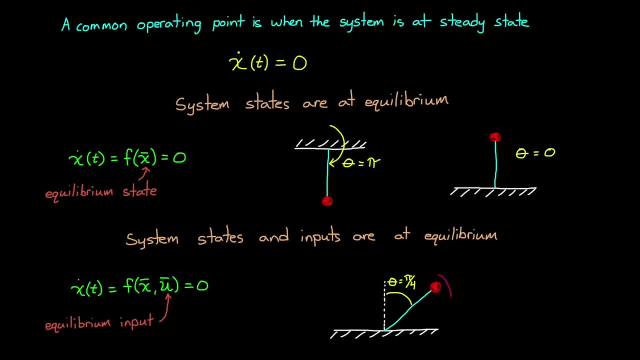 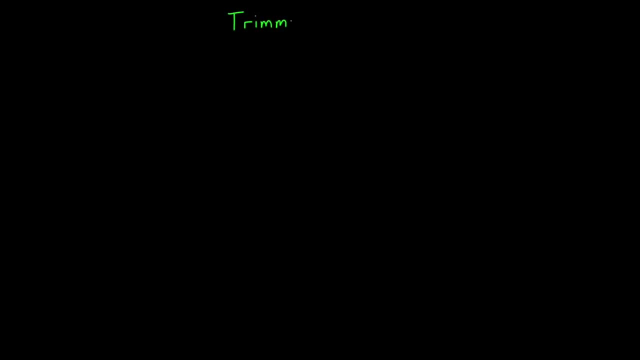 4 radians. If we initialize the pendulum in this condition, it would not move, since the torque from gravity and the input torque perfectly balance out, and we can linearize around this condition as well. Now the act of finding an equilibrium by adjusting the input signals is called trimming, and this is a 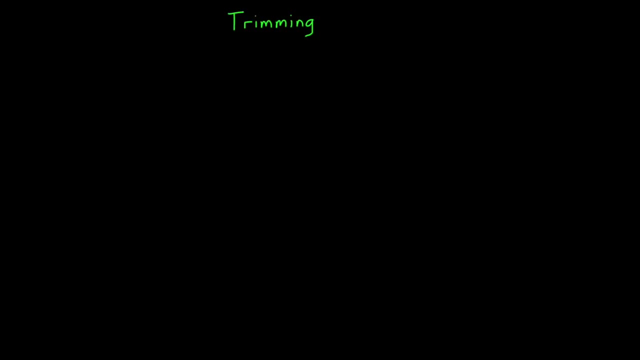 term that's borrowed from aerospace, like trimming an aircraft to fly straight and level. Imagine an aircraft that is set up to hold a constant altitude when flying at a zero-degree angle of at a given airspeed, with no control input from the elevator. This is a steady-state condition for this system. 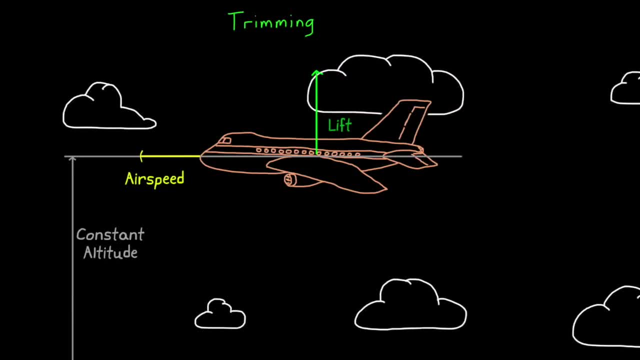 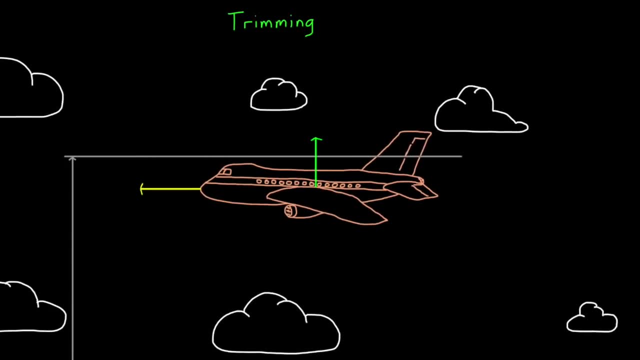 However, if the aircraft started slowing down or was flying at an airspeed lower than the steady-state condition, the wings would generate less lift and the altitude would start to drop. The altitude could still be held constant at this new speed if the pilot added an input into the system. 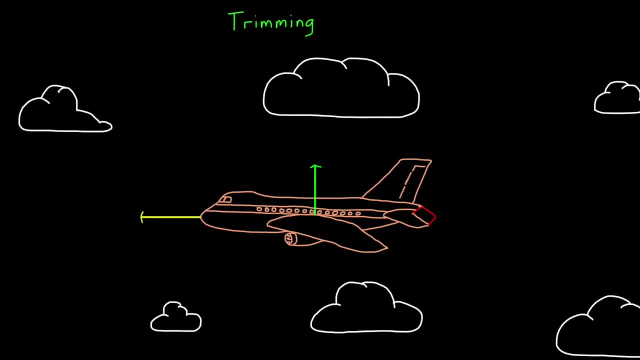 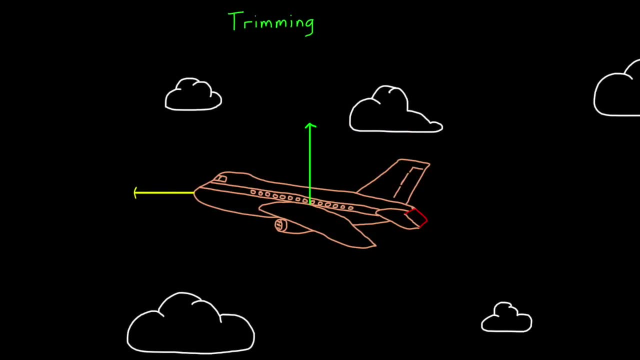 by pulling back on the yoke to deflect the elevator up, raising the angle of attack and generating more lift. But rather than having to constantly pull back on the yoke, the pilot could trim the elevator so that the neutral yoke position produced the needed elevator position that held the altitude constant. 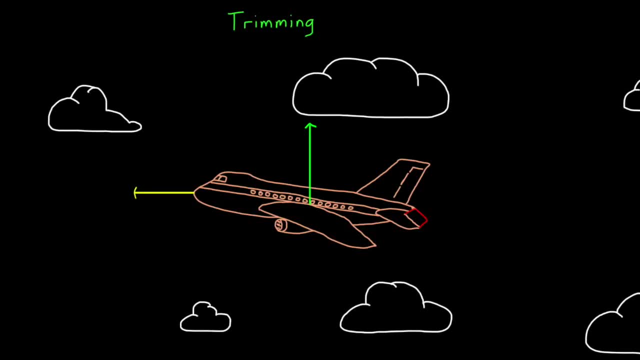 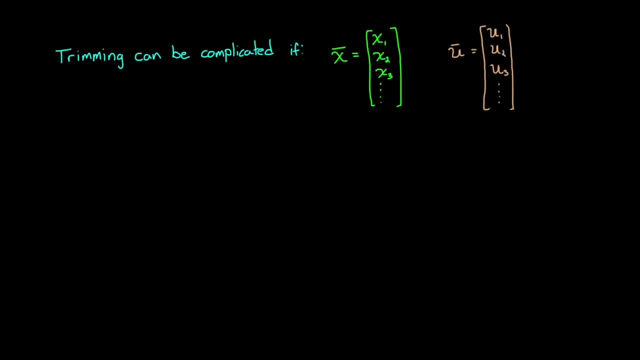 This is what it means to trim: Find the combination of system states and inputs that produce a steady-state situation at your chosen operating points. You can imagine trimming can be a complicated task if your system has dozens of states. you're trying to hold constant and several control inputs that you can use to control them. 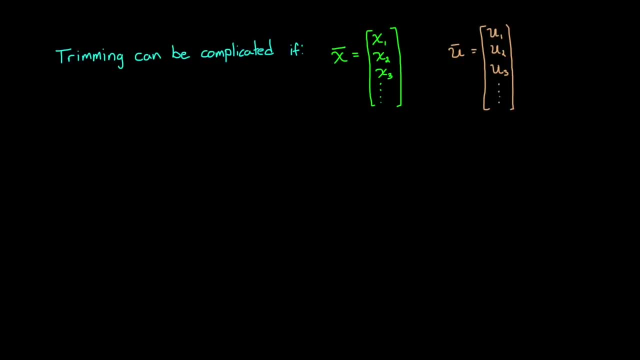 In the next video, we'll talk about some of the tools available within Simulink to make trimming easy. For now, though, it's enough to understand the concept of trimming and how it relates to producing a steady-state operating point. At this point, let me go off on a real quick aside. 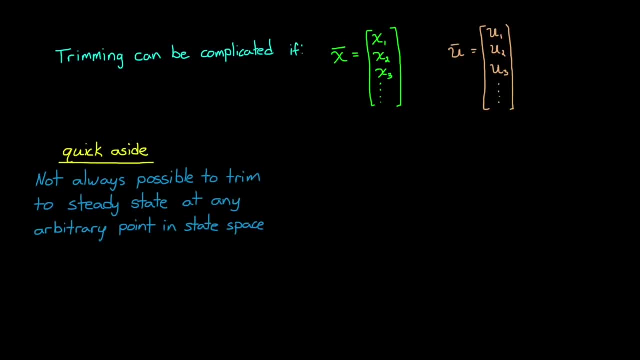 It's not always possible to trim to steady-state at any arbitrary point in the state space. For example, there is no combination of inputs that will cause an aircraft to fly backward steady-state, even though the state space allows for that motion. So you have to understand your system well enough. 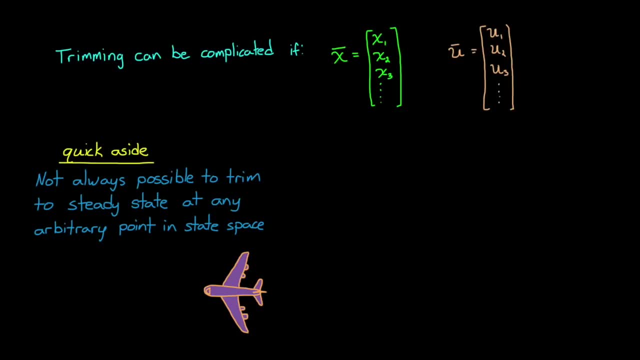 that you don't pick a combination of states that you can't find an equilibrium for. Okay, back to it. We've picked our operating point and trimmed the system so that it's at equilibrium. The next step is to linearize at that operating point. 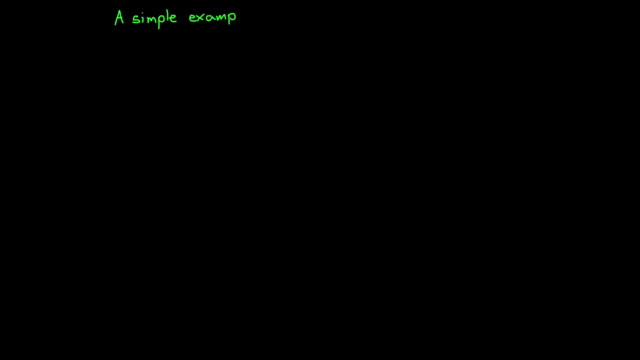 To show how we do this, let's walk through two quick examples. I grabbed this first example from Wikipedia, but I wanted to retell it here and embellish it a bit, because I think it'll give you the basic idea behind linearization and how the math gets simplified. 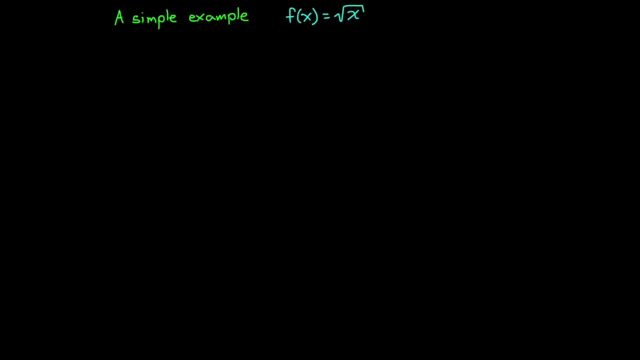 We'll look at the equation F1,. F of x equals the square root of x. Now, this isn't a differential equation, but it'll still help to get the points across. The square root of x is a nonlinear function that looks something like this: 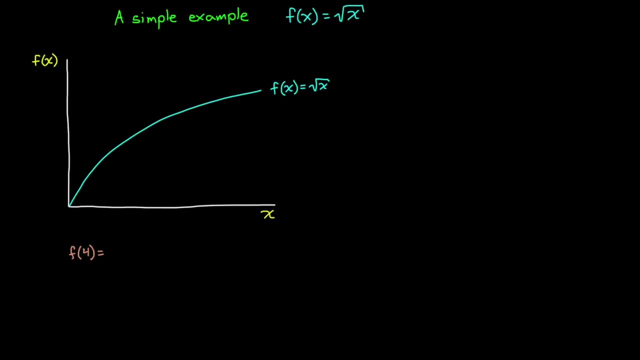 And we may ask what is the value of this function at x equals 4?? And this is pretty easy to solve. We get 2.. However, a harder problem would be: what is the value at x equals 4.001?? It would probably take a fair amount of time. 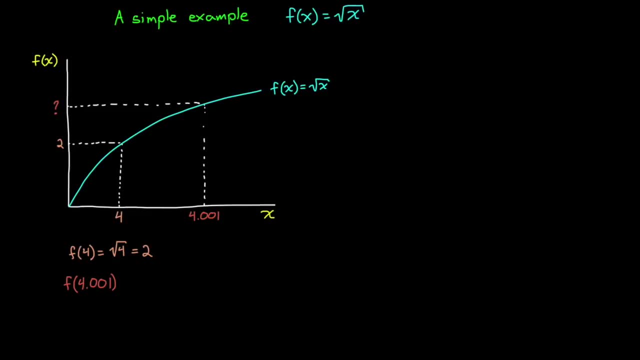 to solve this by hand. However, we can simplify it by estimating the value using a linear equation. The idea is that as long as we don't stray too far from the operating point, then the error between the linear estimate and the true value will be small. 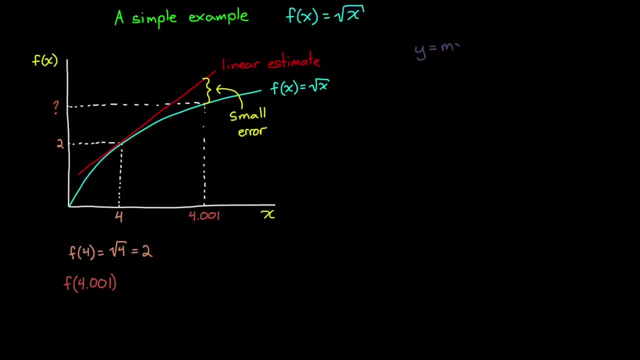 Okay, so let's do that. The equation for a line is: y equals mx plus b, where m is the slope and b is the offset. The slope at any point along the function is just the derivative of the function and the offset is the value of the function. 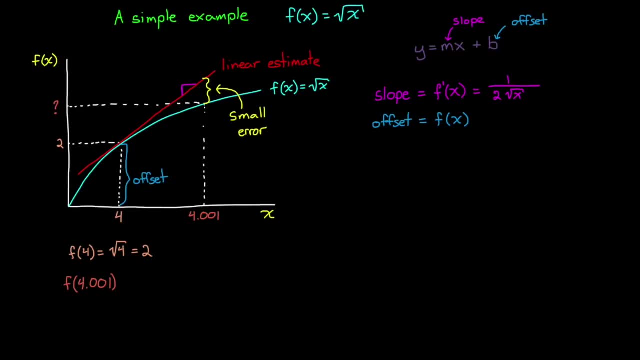 at the operating point. So our linearized equation y of x would be the slope at the operating point, x bar times the distance away from the operating point plus the offset. This is a linearization around x bar and in our case x bar equals 4.. 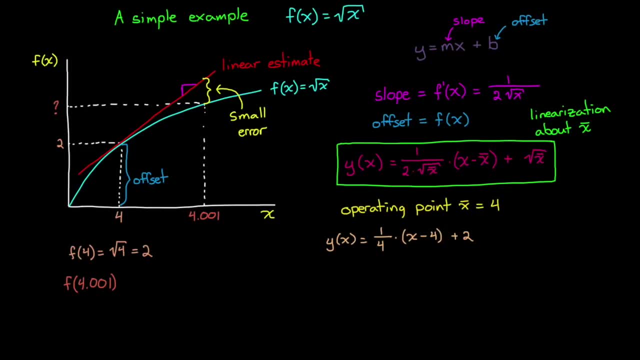 This gives the linear equation 1 fourth times x minus 4 plus 2.. Now we can check the value at x equals 4.001 and easily do the math to get 2.001.. The real function evaluated at 4.001. 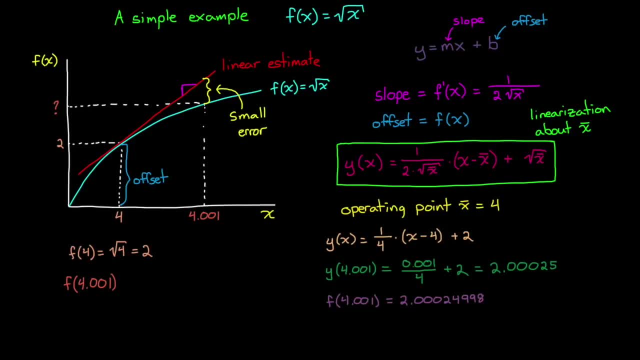 is 2.00024998, and that's less than a millionth of a percent difference. And while it felt like a lot of steps to linearize, we can now use this linear equation to estimate: x equals 4.1 or 3.9. 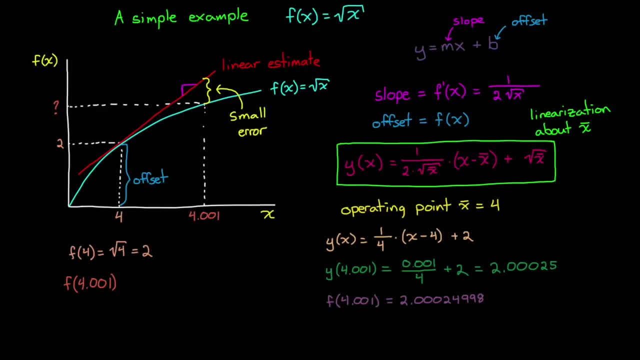 or any number near the operating point quickly and with very little error. However, if we try to use our linear equation at the operating point, at x equals 2, then the error is over half a percent. So if that error is more than we can handle, 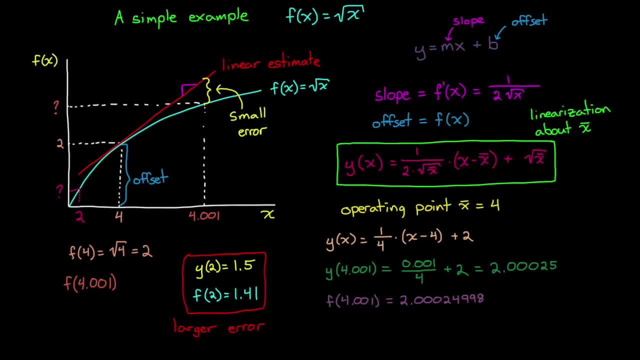 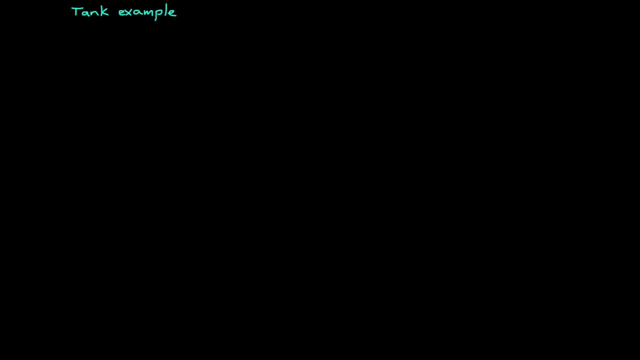 we may choose to also linearize at the operating point 2 and then hand off between the two linear models as x changes between 2 and 4.. Even though this example was simple, it ties in well with our tank example that we started with. 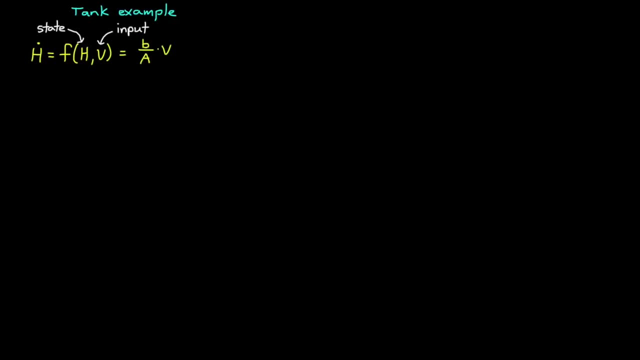 Remember h dot, which is a function of state h and input v was given as this nonlinear equation, So let's linearize it. First we choose an operating point and I'll stick with h bar equals 4 to make it similar to the last problem. 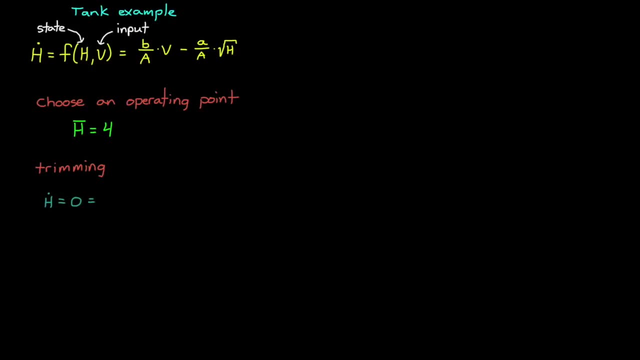 Now we can trim the system so that h dot equals 0 by setting h to the operating point and solving for the input And we get v bar is 2a over b And with these values the function evaluated at the operating point equals 0.. 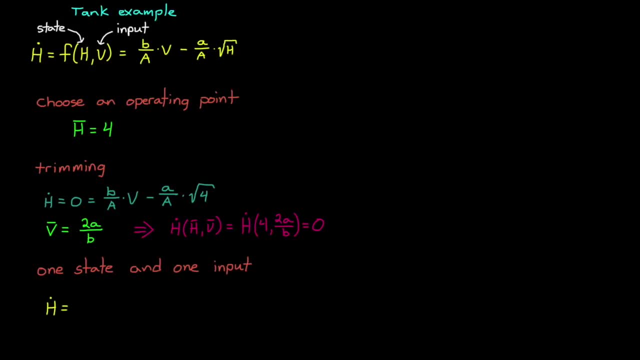 Now, this system only has one state height and one input voltage, So we can expect the final linear equation to be in this form, where both matrices are 1 by 1.. All right, now that we have a trimmed system at the operating point, we can now linearize it. 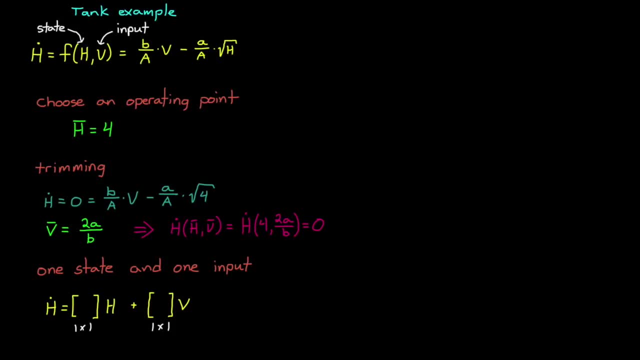 And I want to remind you that what we did before was replace the function square root of x with a linear line. y equals mx plus b. We're going to do something a bit different here, but the result will be very similar. We're going to expand our differential equation. 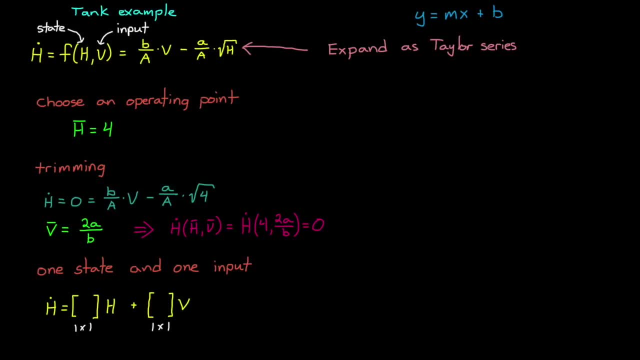 with a Taylor series, But instead of keeping all of the terms out to infinity, we're going to ignore all of the higher order terms. In this way, we'll only keep the zeroth and first order terms, or the first derivatives of the Taylor series. 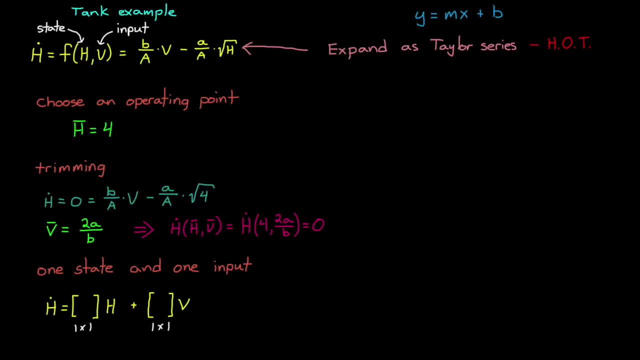 Now, the math involved in this is more than I want to cover in this video, But my goal is really just to give you an idea of how the derivative of a function can be used to generate a linear approximation And, if you work through the Taylor series, expansion and remove terms. 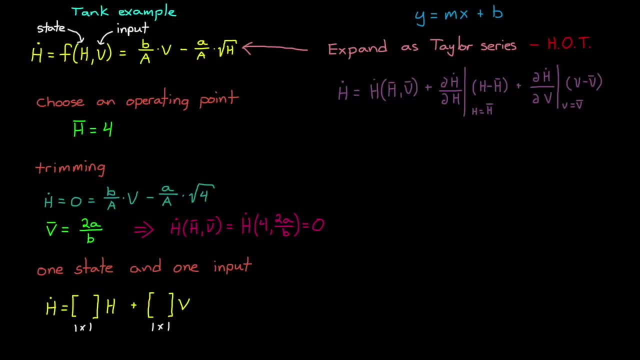 you'll be left with the following function. And look at this. It bears a striking resemblance to: y equals mx plus b. We have the offset, Or the starting point of the function, which is just the value of h dot at the operating point. 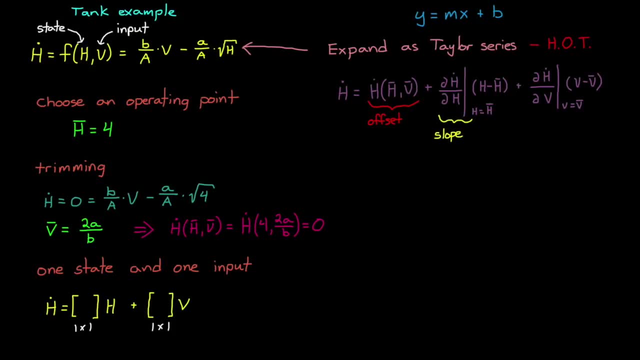 And then added to that is the slope of the function as it relates to the changing state, multiplied by the distance the state is away from the operating point. So this first addition takes care of the changes due to changing state and the second addition takes care. 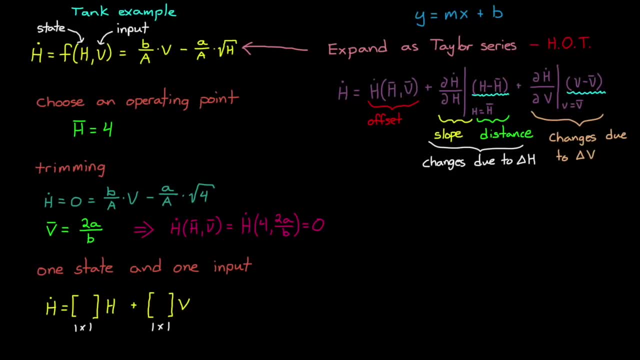 of the changes due to changing input. But we can simplify this further, since the function's value at the operating point is zero. Now we can solve the partial derivatives And to simplify this result even further, we can just relabel where we call zero. 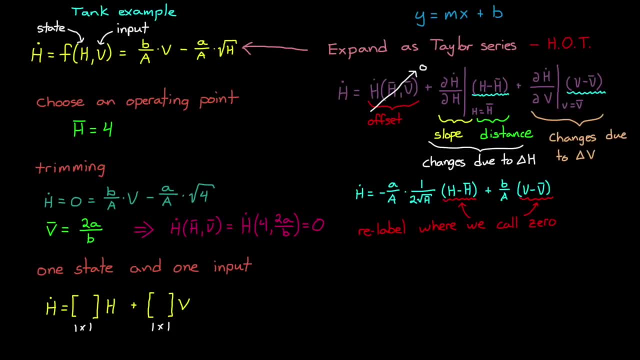 So instead of the height being measured from the bottom of the tank, for example, we can measure it from the operating point, And this condenses h minus h bar down to just h and v minus v bar down to just v. And what we're left. 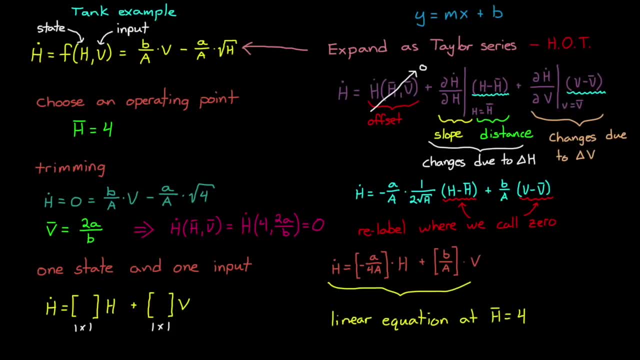 with is this linear equation of our water tank system at the operating point four. And just like with the previous example, as we stray from this operating point, this linear model will behave less like its nonlinear counterpart. And if we can't handle that error, 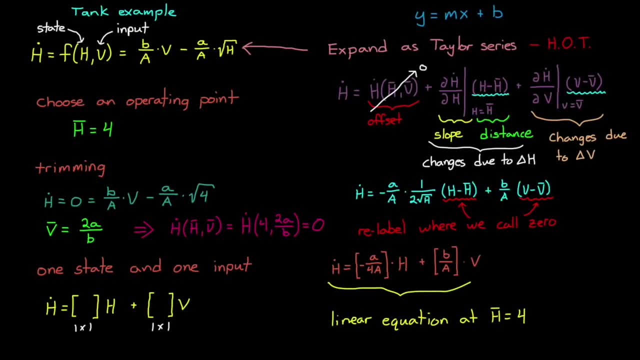 then we would just linearize a second time at a new operating point. When you have multiple linear models, you can develop a linear controller for each of them and hand off the control gains from one region to the next. This is the idea behind gain scheduling. 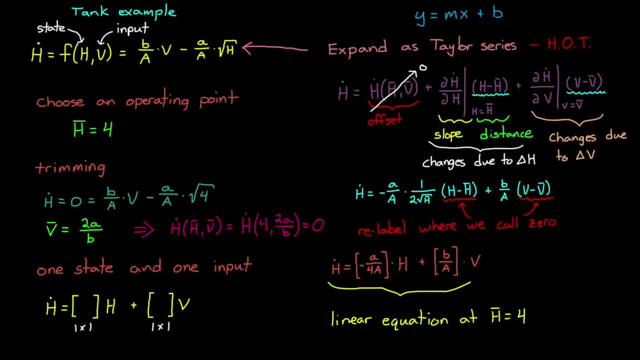 and I've linked a video in the description on this topic if you're interested in learning more. There is also a link to the Water Tank System, water tank model linearization example and math works page to learn more about linearization of Simulink models. so I hope you check them out as well. what we 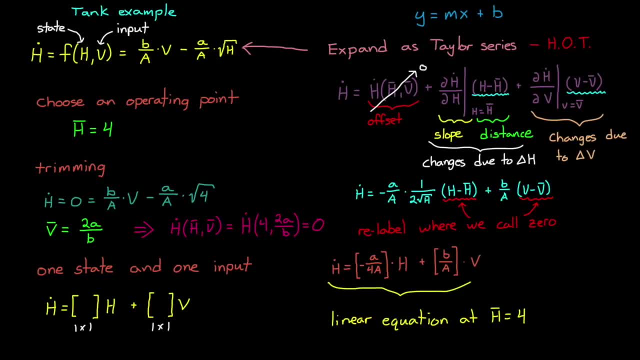 did here was Jacobian linearization. we built a linear model by looking at the first-order derivatives of the system, and this type of linearization requires the function be differentiable at the operating point. but there are other linearization methods as well, and in the next video we'll explore some of those. 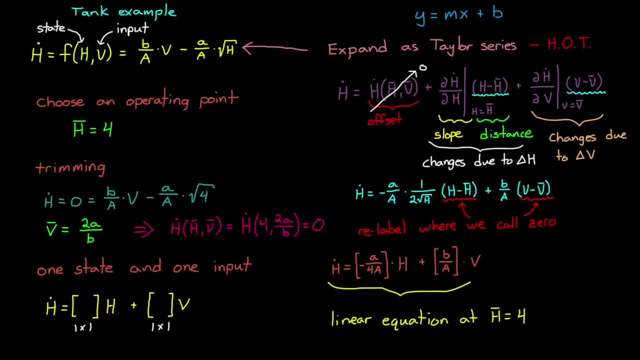 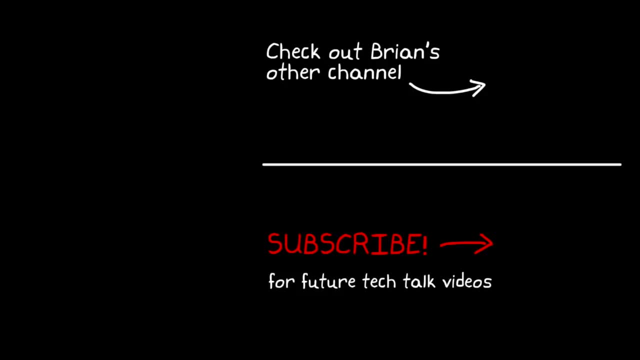 other methods, what tools exist for them and how to understand what they're doing under the hood. so if you don't want to miss the next tech talk video, don't forget to subscribe to this channel. also, if you want to check out my channel control system lectures, I cover more control theory topics there as well. thanks for watching and I'll see you next time.